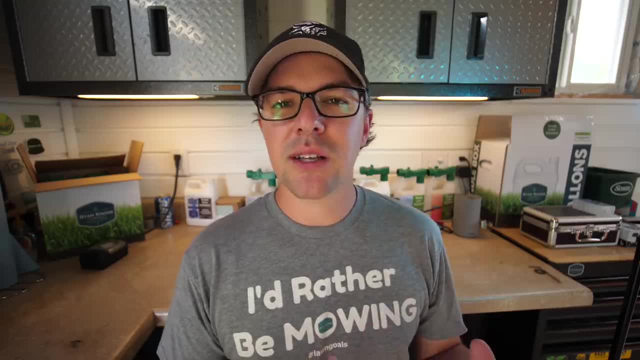 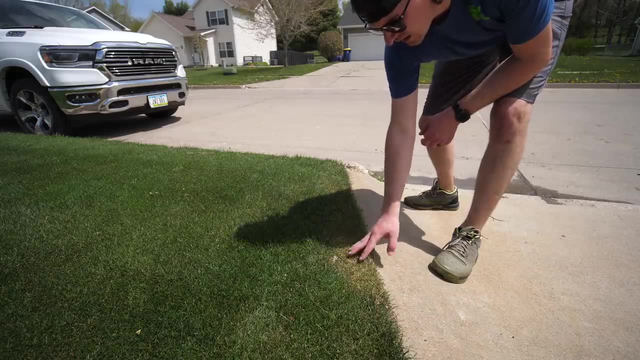 at- That's probably the easiest way- or just watch when it's about to get to the wilting stage. and what I mean by wilting is you'll start to see some of those hazy, bluish type spots in the yard where it's just starting to wilt over the grass blades. That's the time frame when you know that you need. 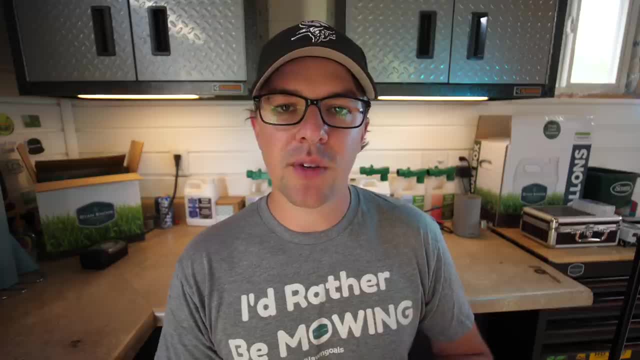 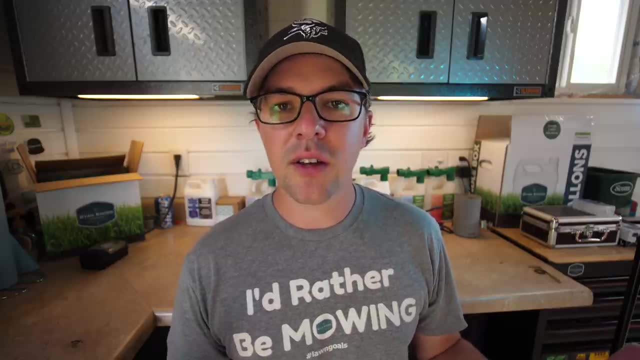 to get some water on the turf. Another thing with watering and irrigation that a lot of people don't think about is that if you have just a few spots here and there that need some water, you don't have to water the whole yard. If the rest of the yard is looking good, just start to get those spots with. 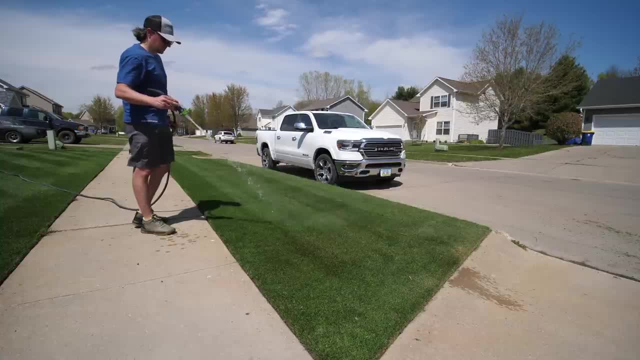 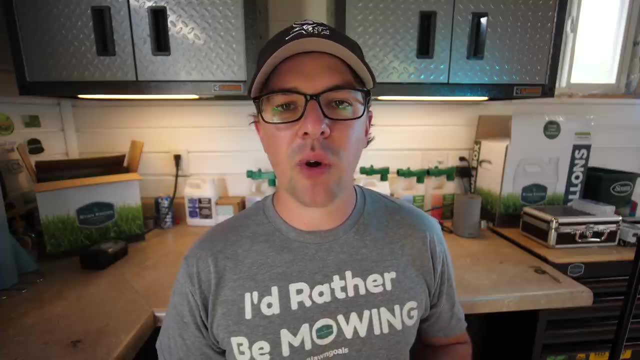 some hand watering and a lot of times it can keep things going for longer and also conserve some water as well. So proper irrigation, factoring in your rainfall and the humidity in your area, that's step number one. So step I would say 1a is also: you could look into some wetting agents. So what? 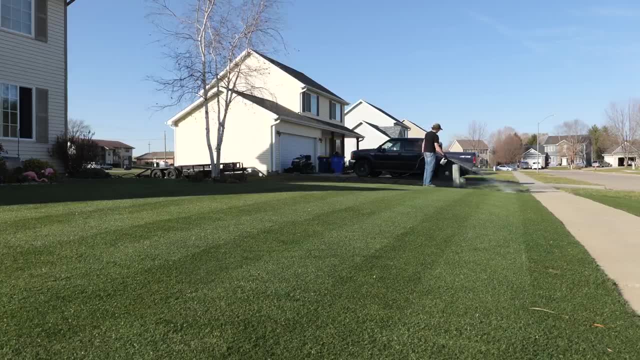 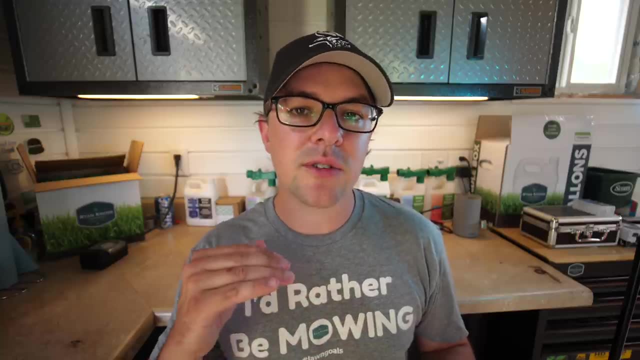 they're going to do is actually help your water to soak into the ground properly, especially when it gets dry here on our soil it'll get sort of a crust on the top of it and a lot of times during dry parts of the year, you can watch the water absolutely just run off of the soil. What these 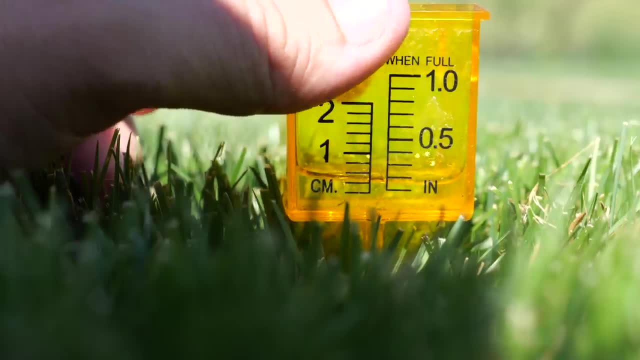 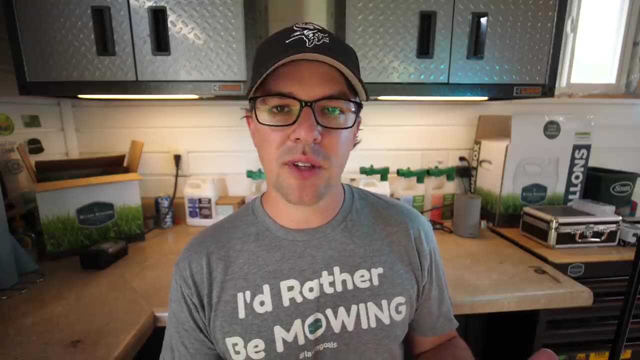 products do is to help that soil become less hydrophobic so the water actually soaks in and goes down and is used properly. Wetting agents is another thing. it's a whole deep dive topic. it's not something you absolutely have to have to keep a green yard. 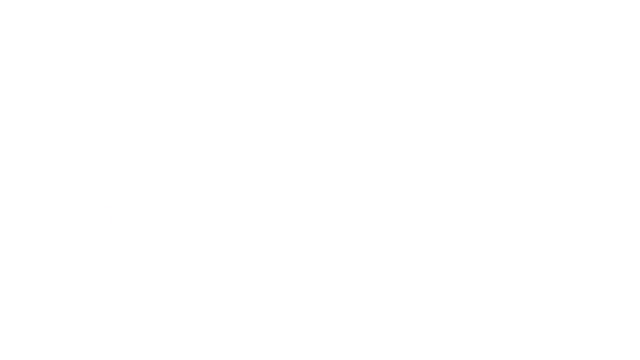 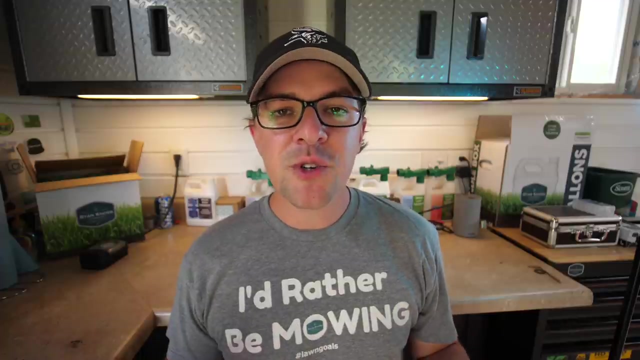 but if you are interested in going the extra mile, check out some of those products. Step number two on how I continue to keep a green yard during the summer is I continue to fertilize. A lot of people might say I thought you weren't supposed to. 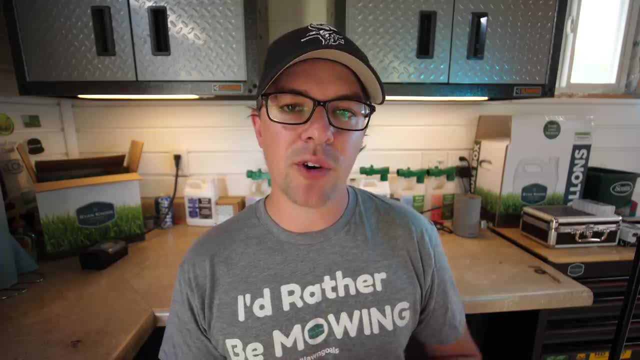 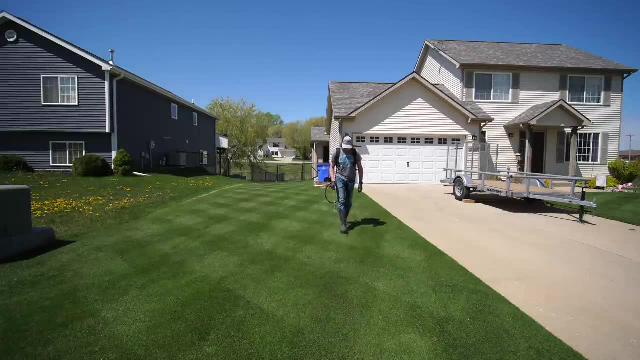 fertilize cool season lawns during the summer. I'm really always on a low-key program on my low-cut turf, where I'm applying a lot less product but more often, but this is something that you can apply to any yard, as long as you're watering during the summer by applying just low amounts. 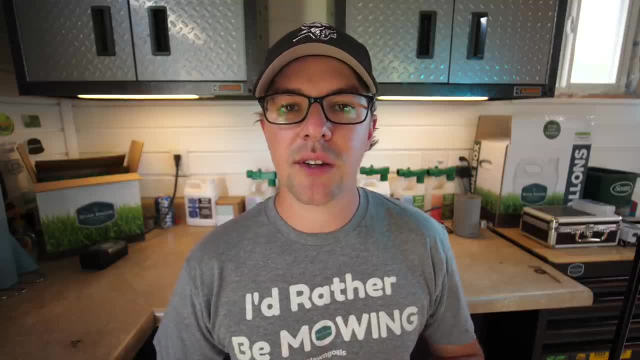 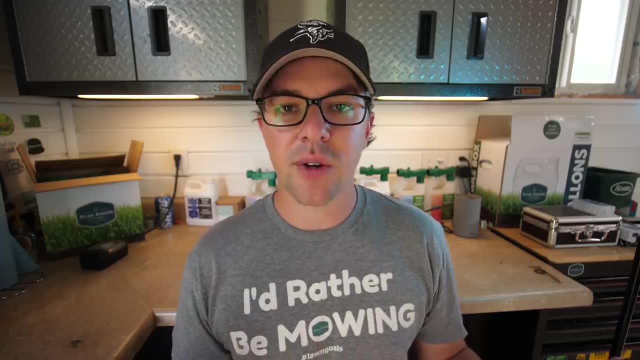 of fertilizer and micronutrients to your lawn to kind of keep things green and going. So a lot of times if you're on a four-step program like a granular program- the middle summer piece, there is something where there's not really any fertilizer going down and your spring application. 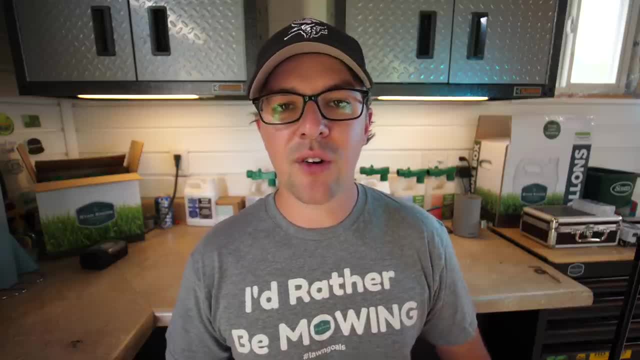 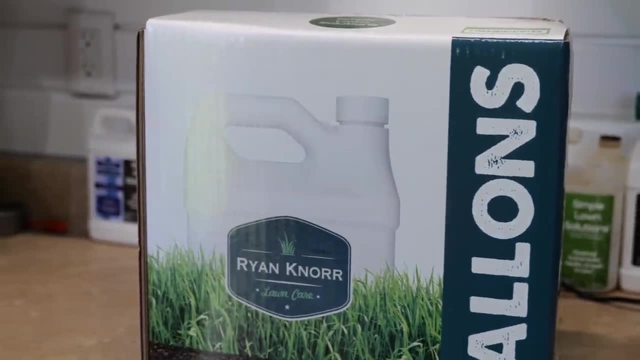 has to last you all the way until fall. For a lot of people that's fine, but the thing that I found in keeping a really green and nice looking lawn in the summer, in addition to the irrigation, is to continue those low doses of fertilizer. So right now is a perfect time. 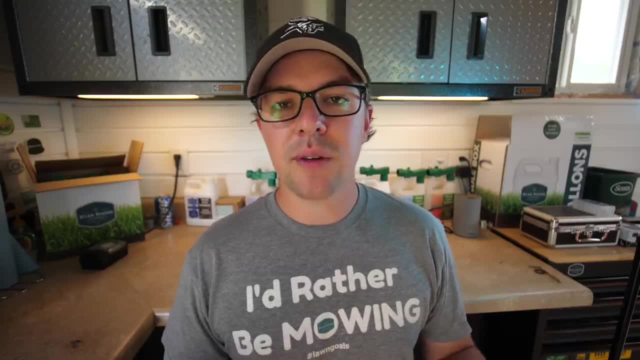 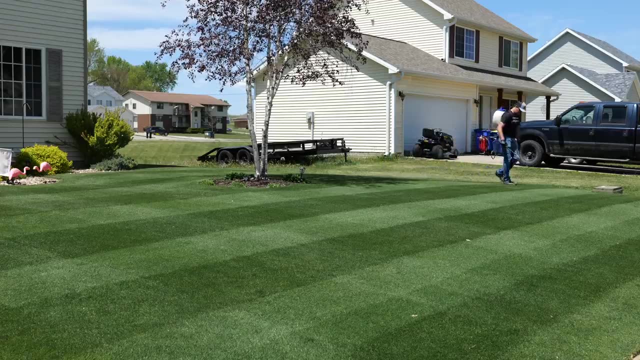 to start doing that, and this is a great way to get those low doses of fertilizer out of your lawn, because the liquids work really well for this. Granulars can work as well if you can put them out at low doses, but a lot of times it's hard to do that in a spreader. Liquids would be what I. 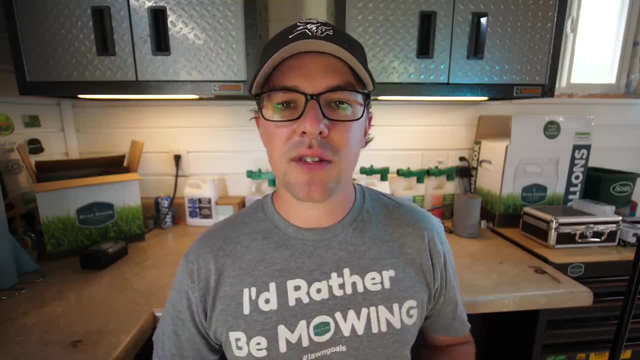 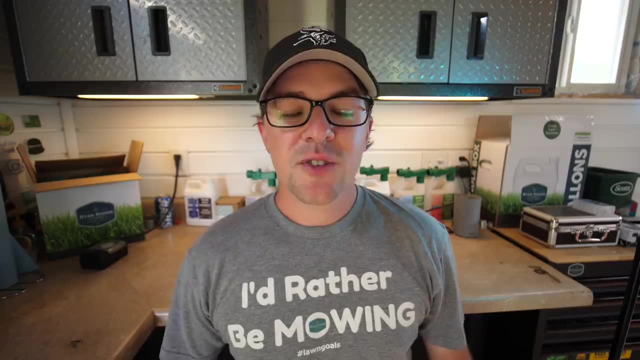 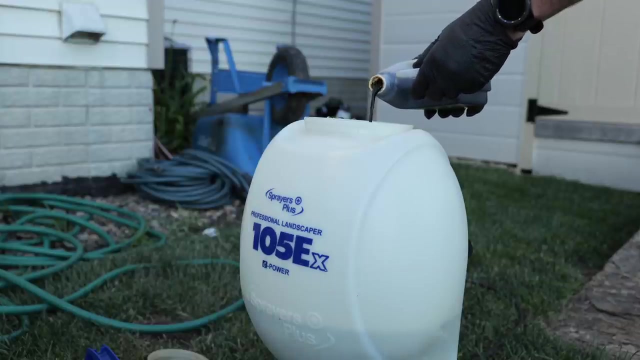 would use in order to put out a low amount of fertilizer- you won't cause any extreme growth- and utilize these to give the lawn some nutrients, keep it green during this summer period. Step number three is related to that fertilizer, but this is specifically iron and other micronutrients. This was something in my program that I didn't do a lot of at the time. 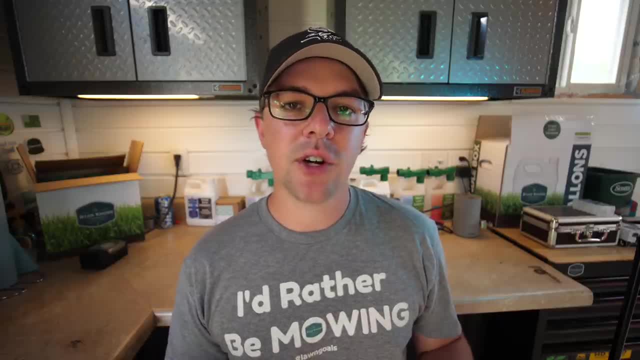 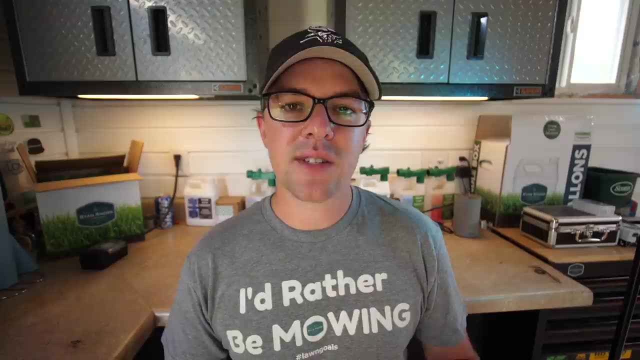 the beginning, and since I have done that, I've noticed a major difference in terms of keeping my lawn green during the summer, keeping it green during the stressful parts of the year. Specifically, a low dose of micronutrients every two to three weeks is what I'm on for my program. 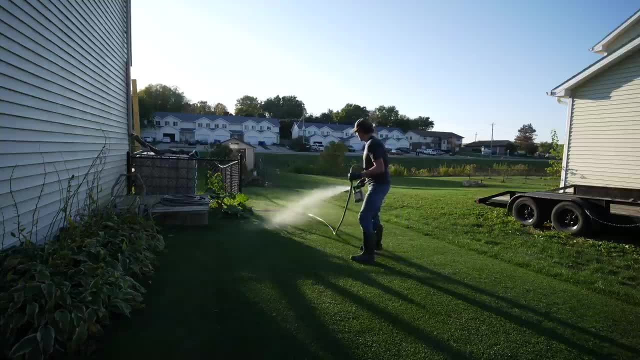 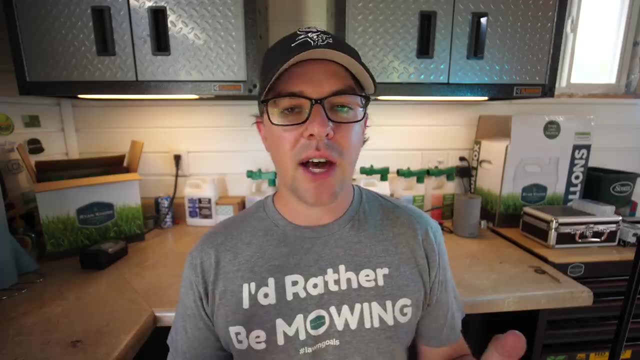 Again, these are small doses that you're putting out, but they do make a big difference in terms of holding your color throughout those stressful periods and throughout a time frame when a lot of other people's yards will kind of go off color. There's a lot of different products on the market. 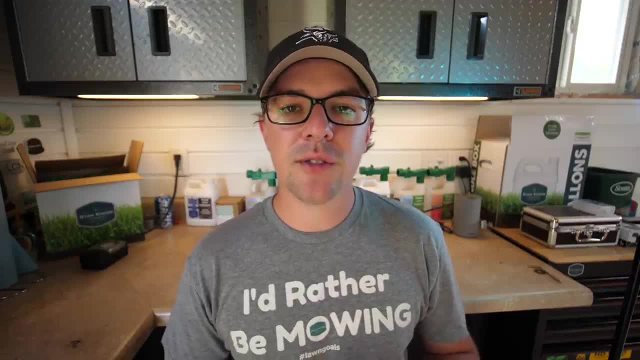 I will list a couple in the description if you want to check those out on what I personally use. but iron and micronutrients are a great way to keep your lawn green throughout the summer. The micronutrients are a way that I keep my color going during the middle of the summer as well. 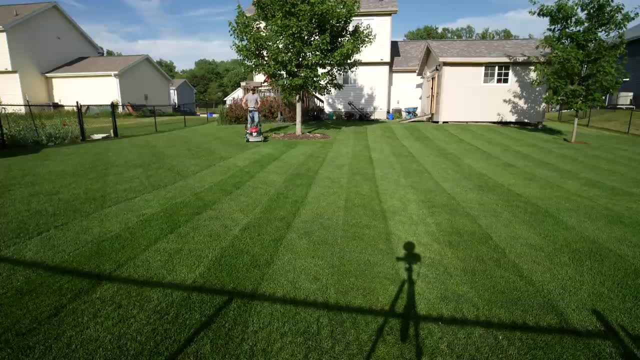 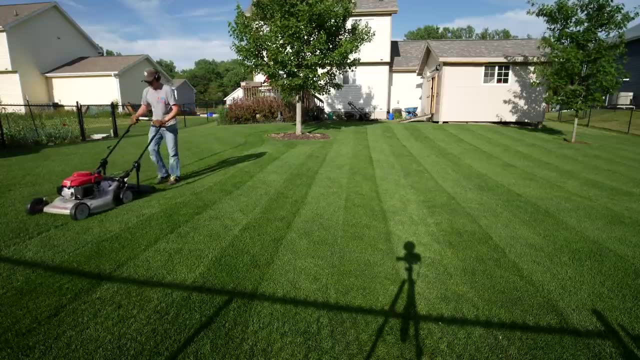 Next step would be proper mowing and sharp blades. I talked about this in a previous quick tip video that if you're not mowing properly and at the proper height, you're going to be causing a lot of stress to your lawn, and especially during the stressful period of summer for cool season grass. 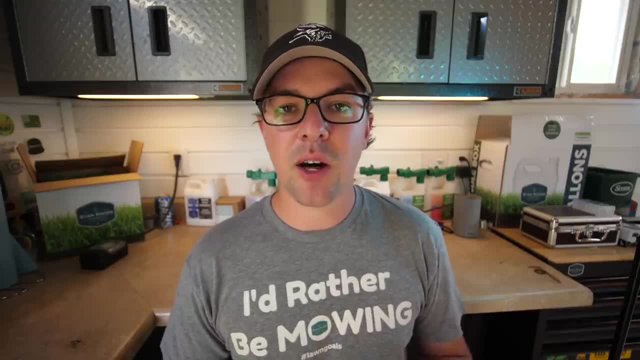 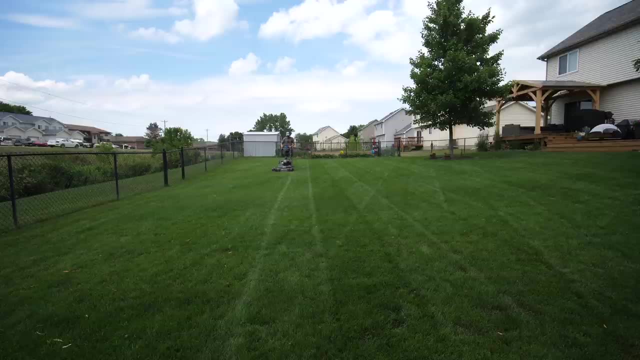 it's going to look really brown really fast if you're stressing it out by scalping. So make sure that you're properly mowing at whatever height you want to be at. that means you can cut it low, like I do, if you're willing to mow more often or if you're one of those once a. 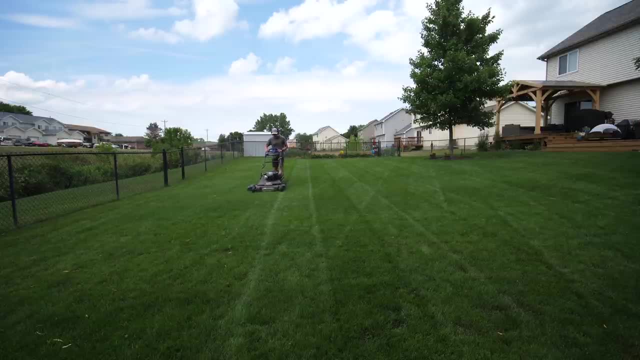 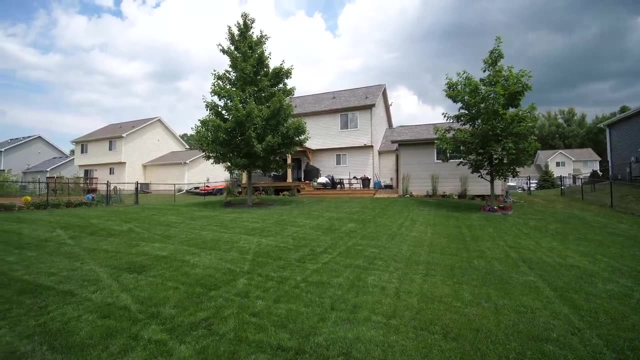 week type people, I would probably have it at least three inches during the summertime. That way you're going to be causing a lot less stress when you do mow the lawn and the growth is going to be coming down. so if you don't need to mow that often, you want to let it get a little shaggier during the 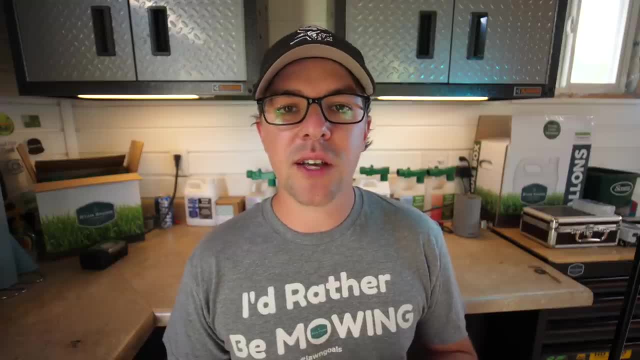 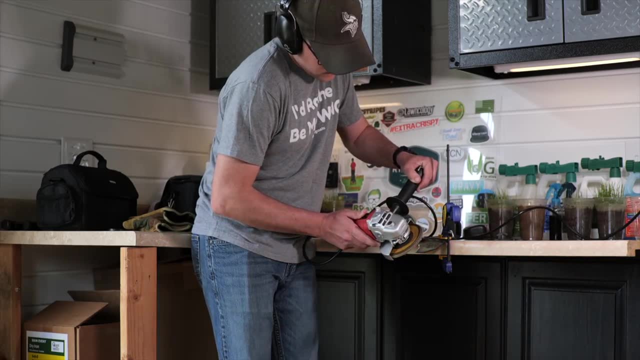 summertime, that's totally fine too. Make sure that whatever mower you're using, it's working properly. you have your blade sharp. this is going to give you a lot more success as well. make sure your equipment is working properly and you're cutting those grass blades as clean as possible. And finally, 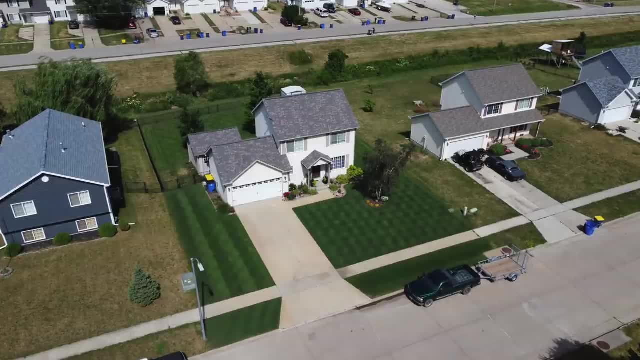 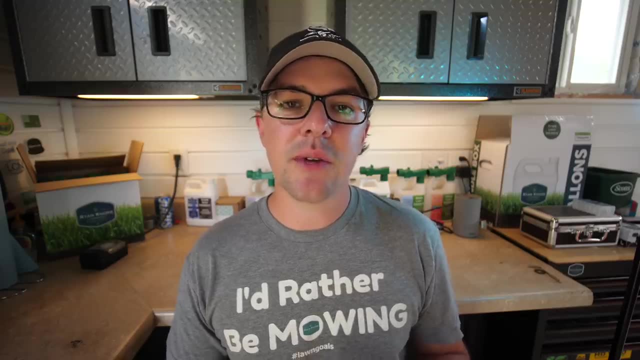 when it comes to a green lawn like the one I have a lot of people tell me. I've applied a lot of different things, Ryan. I've done so many different practices and I can't get my lawn to be as green as yours is. There's also a strong likelihood that people aren't thinking about grass cultivars.